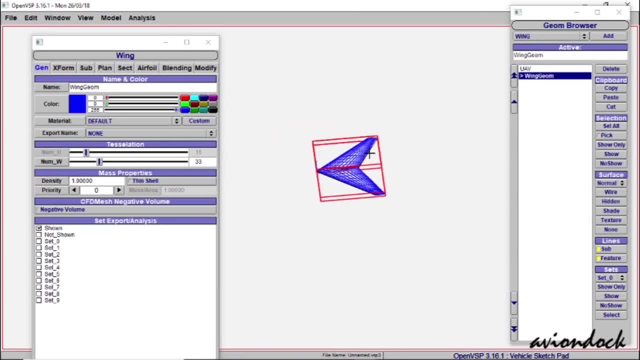 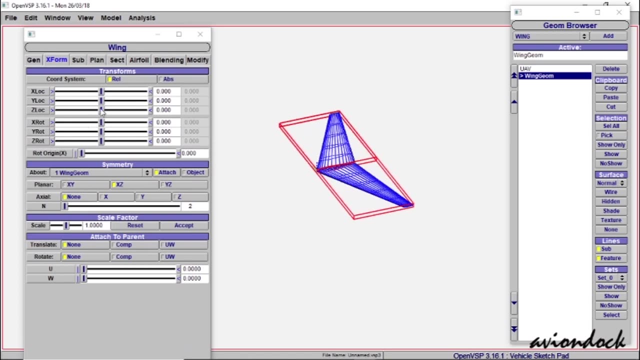 this wing is fully parametrized. I don't have to create a wing like you would do in other default CAD softwares. So here under the wing section, we have the rotation and the translational features, So I can change the XYZ location and now, in this current orientation, you have the leading. 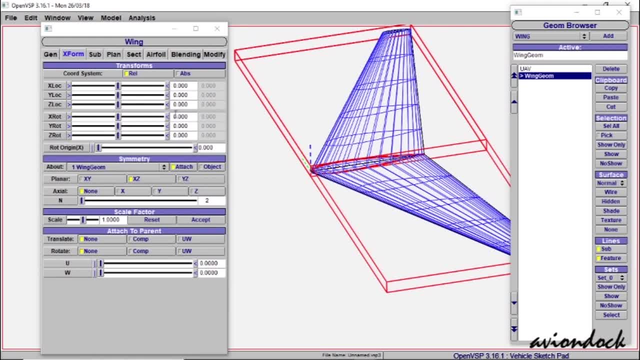 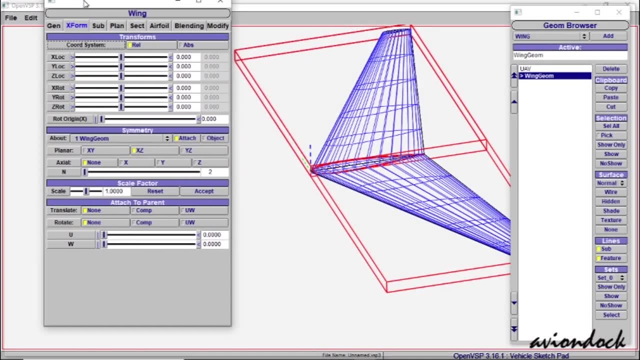 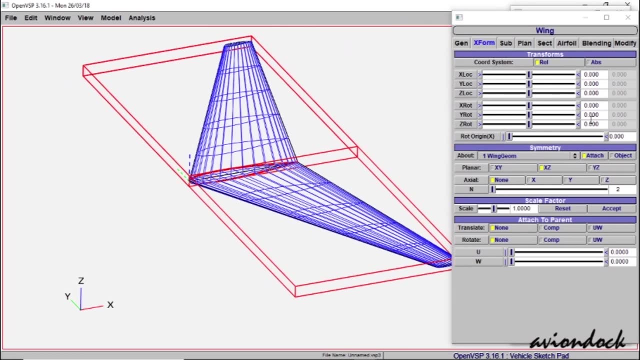 edge of the wing, at the origin of the coordinate frame of reference. You can also see the frame of reference at the lower left corner of your screen And next we have rotations. So the rotations are useful if you want to make a vertical tail or add anhydril or dihedral. 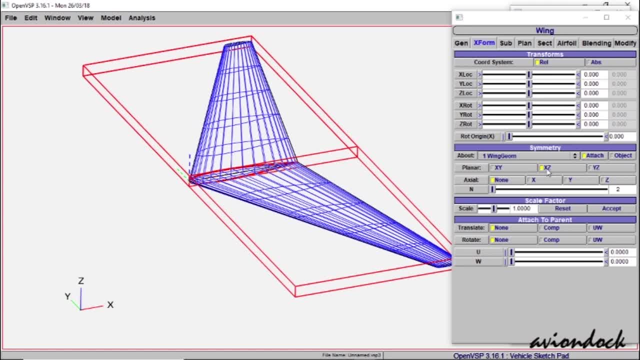 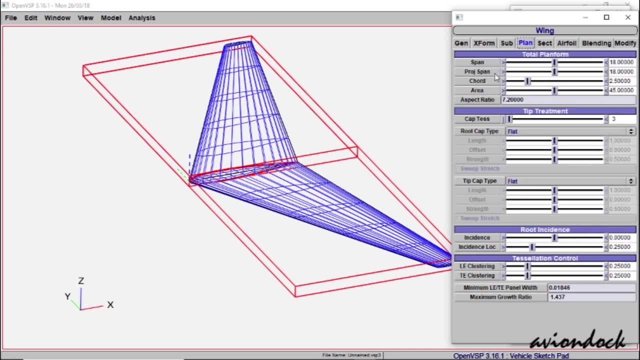 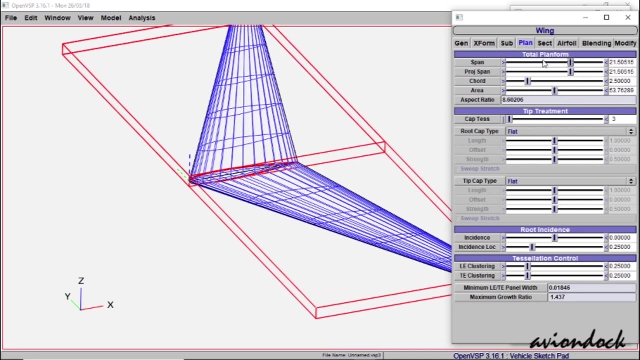 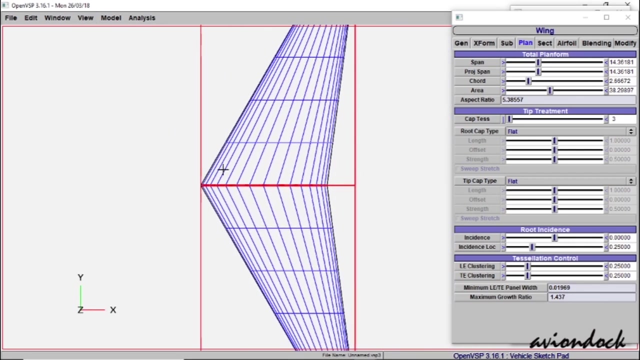 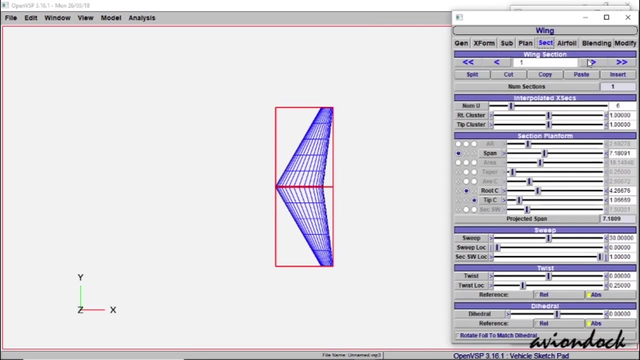 to your aircraft model, And so we see in the subsection: let's go to platform and here you see the most common variables associated with a wing design. So we have span that can be altered, and also the area. Just go to top view. So we have in the section- we have multiple sections. 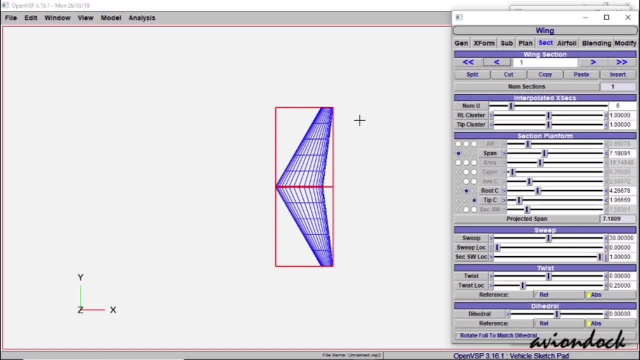 And so currently this is just one section. So if you want to have a multi panel wing, you can cut this into two sections or more than that. So if I put split and then now I have two wing sections and I can independently control the span of these sections. So that's. 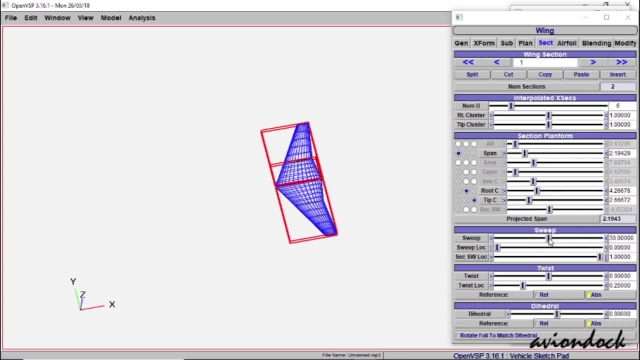 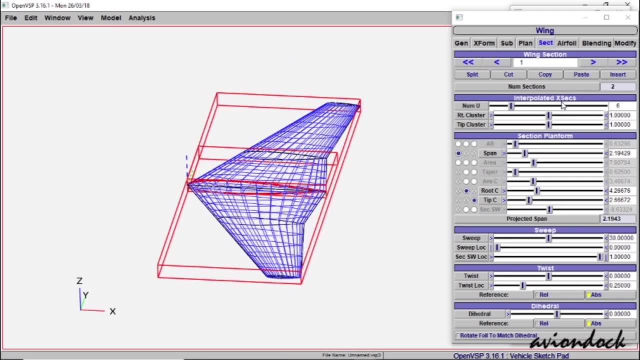 how I control this. And then we have the other features, such as sweep, the location of sweep and also the twist required along the span of the wing. So let's leave this wing as it is, since this is more of a quick run through to how. 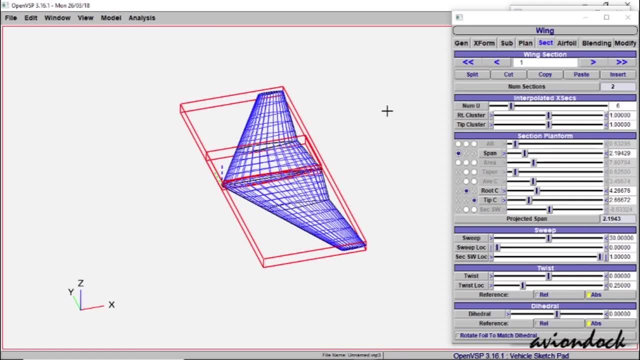 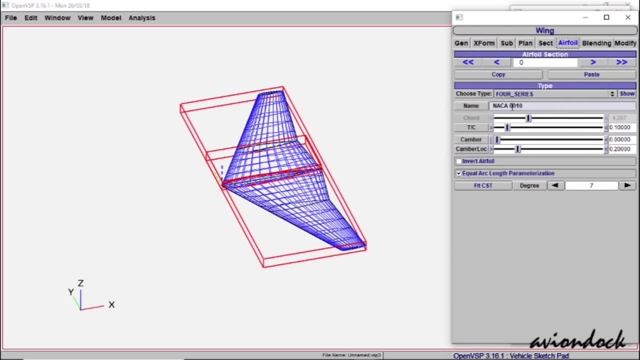 to get up and running the aerodynamic analysis on a configuration. Next we have the airfoil section. so here we can either define your 4 series NACA airfoil, so let me just change this from the symmetric configuration to general wing airfoil. so 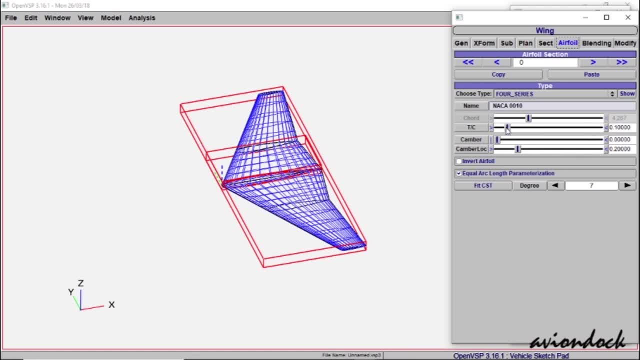 let's use the 2412, so that's how I can change this. I can change the thickness to chord ratio, which is the last two digits of the NACA airfoil, so I can directly change it here and the camber. so that's the camber as the first. 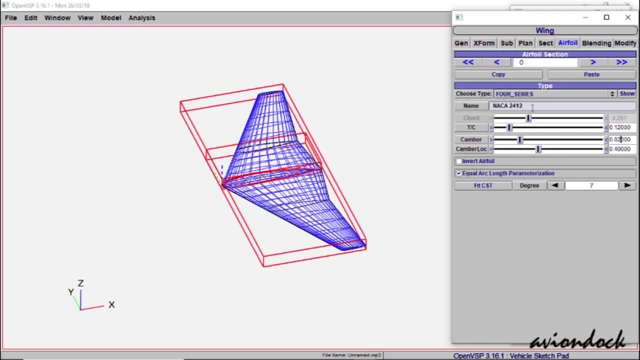 and the camber location is the second. so I have NACA 241 to define and then we look at the airfoil cross section here. that is alright. So if you're interested, you could have different airfoils at every section. so let me define this NACA 2412 at all of these sections. 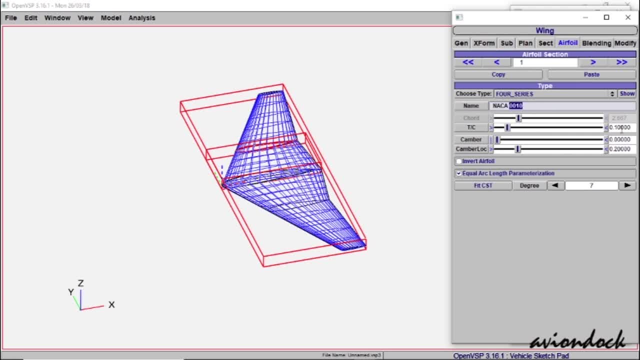 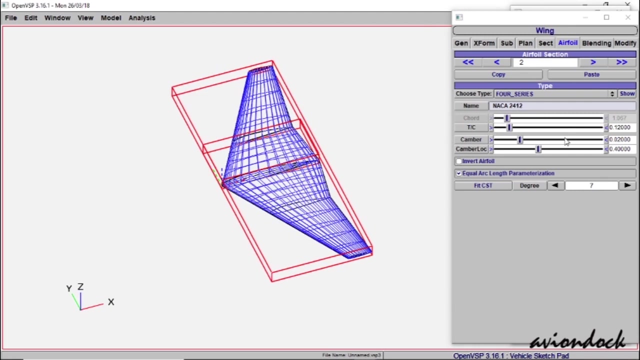 This should be 4 and 2,. sorry, I need to remove these two. Alright, So, So we have 2412 at section 1, alright, so we have all of the sections of the wing defined with the same uniform airfoil. so this is a non-symmetric airfoil, and so that's how. 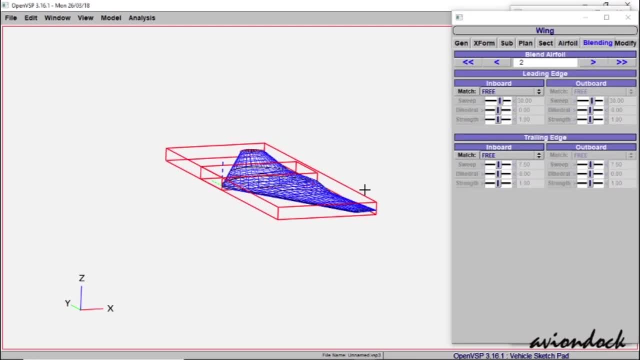 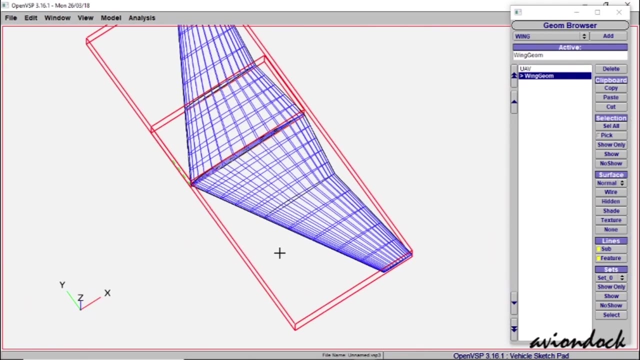 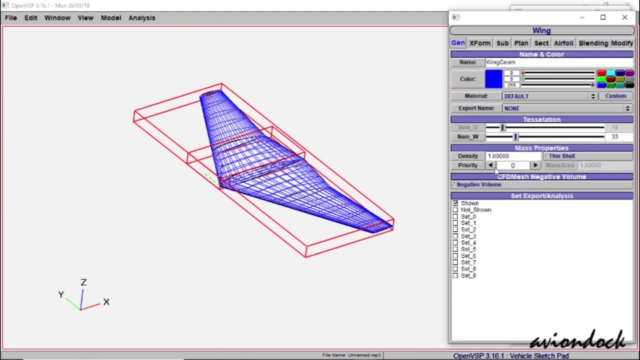 we have our wing. These are other features. This is to have additional spanwise components added to the wing, such as winglets and things like that. so let's just leave it at default and we close the wing. So in the wing. one thing we missed was also in the general, you could define a density. 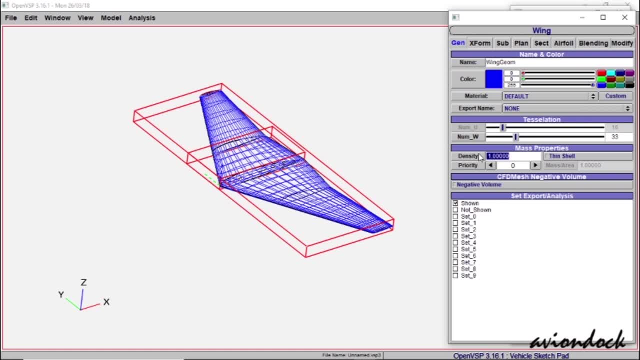 for your wing. so if it's made from composite materials or aluminium alloys, you put the right density. So this step would something that would be something of interest for us to be used later in a structural calculation or a stability analysis where we would be requiring the 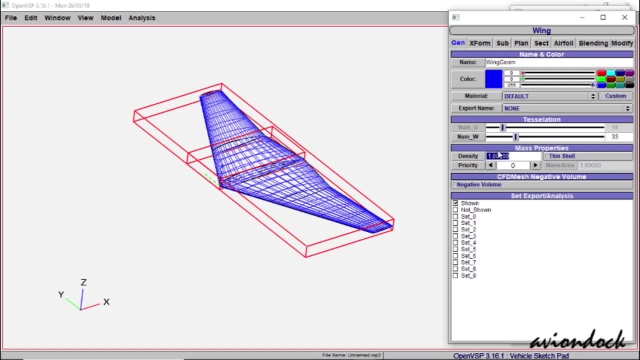 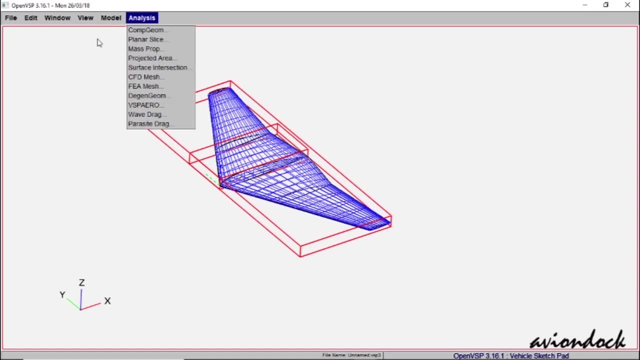 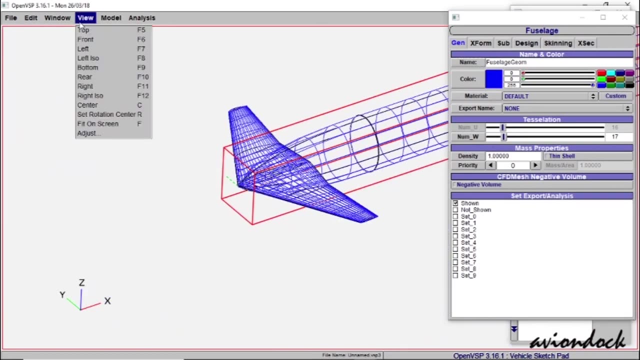 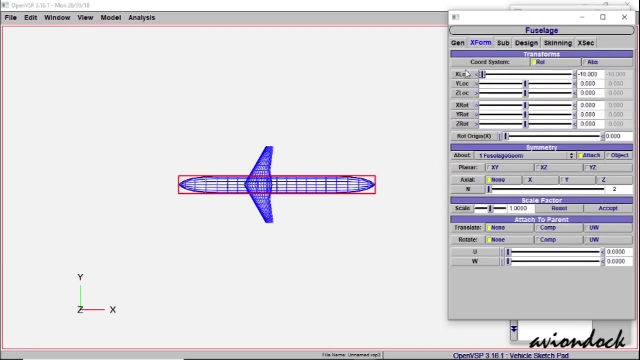 inertia of our configuration, So I leave this as a default of 1.. Alright, so let me quickly add a fuselage. So there, we have the fuselage, Alright, So, And so let me scale down the fuselage. I change the x coordinate position and also I can. 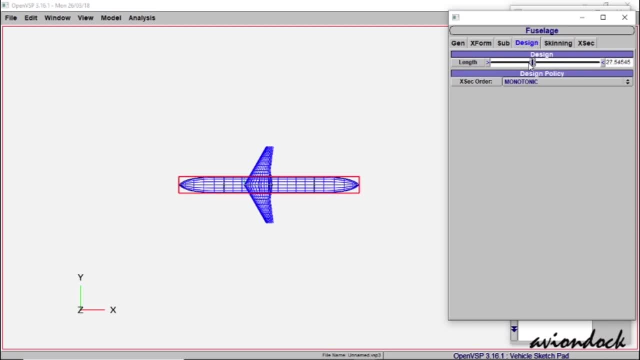 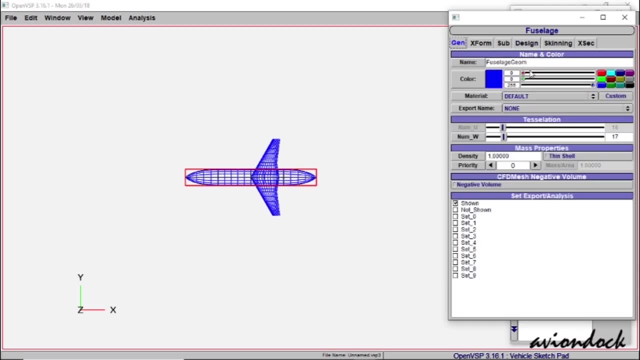 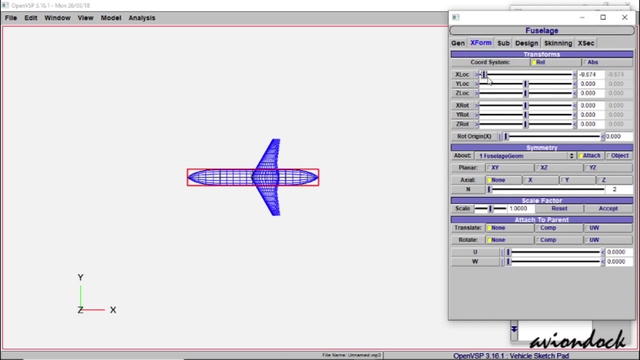 go to design and reduce the length of the fuselage. So there's no worry, if you run out of this slider, which has a maximum limit, You can manually change the values here. So let me just bring to an appropriate location. This is nowhere a aircraft that is sized correctly or based on any predefined requirements. 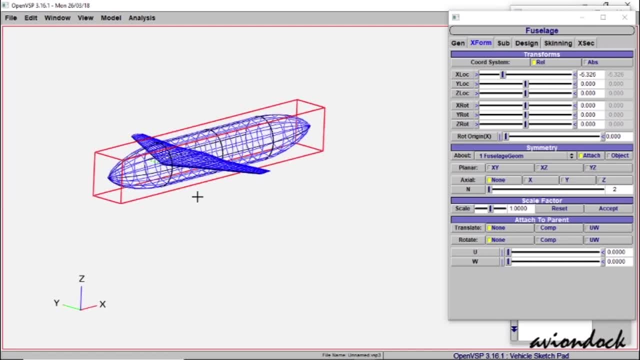 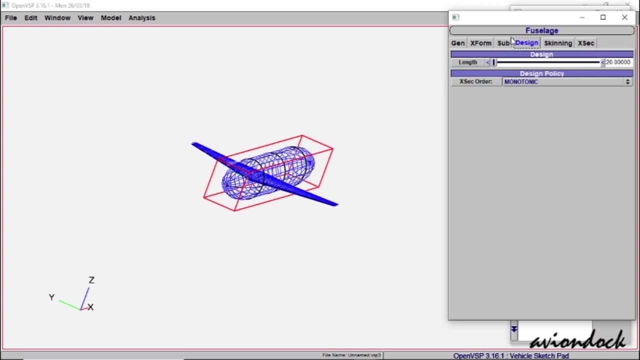 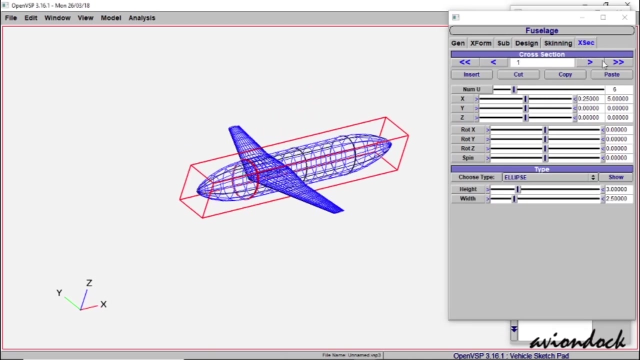 but just a rough configuration that might or might not fly. So we see that the fuselage diameter is a bit too large. Let's try in a, let's see, Let's try Reduce it. So if I go to the x-sections, so that takes me through various cross-sections of the fuselage. 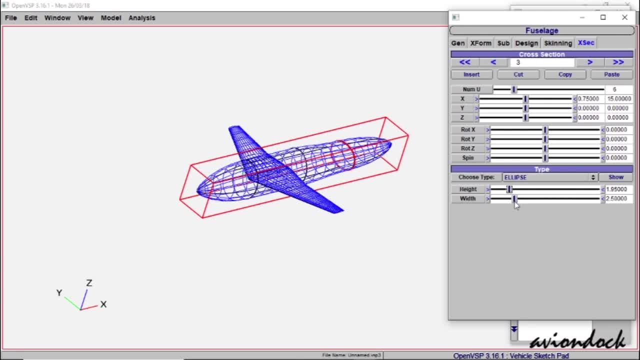 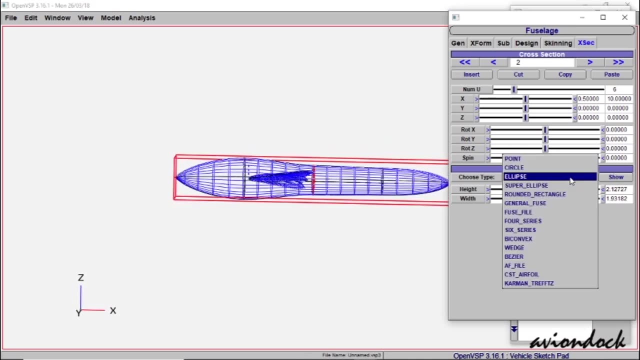 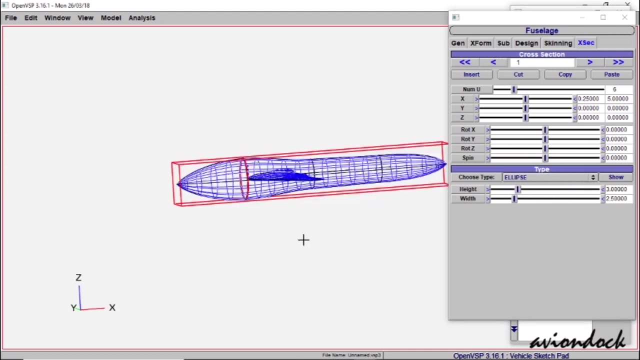 And here I can change the height and the width of the fuselage, So that's an interesting parameter that you can play around with. You could also change the cross-section to a different type, So let me just change the z-location of this a bit low. 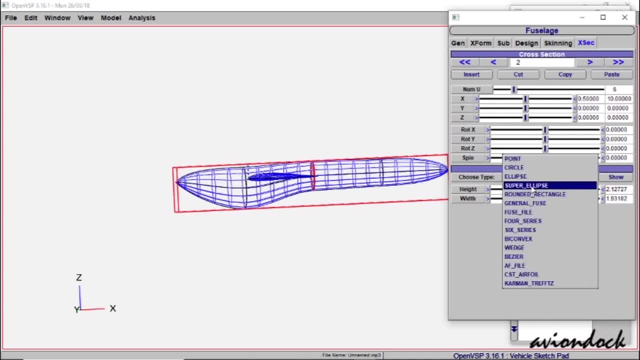 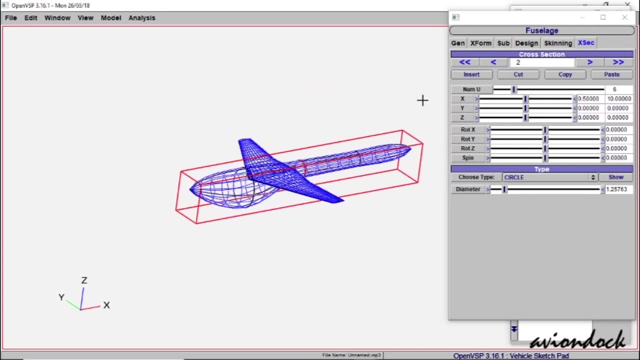 And also change this to a circle, The next one to a circle, Reduce the diameter so that it looks similar to the boom of a conventional fixed wing UAV, Probably move the. So let's say I want to make the nose a bit more aerodynamic. 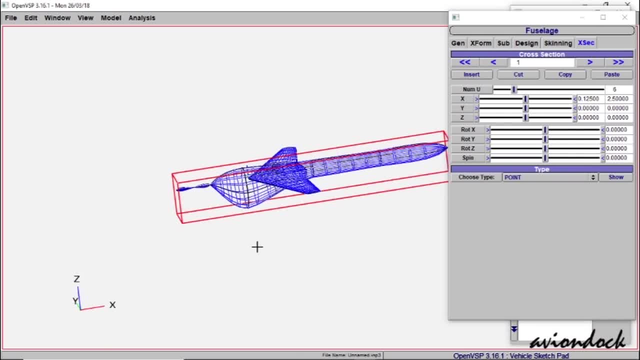 So I can just insert An additional cross-section that I can play around with and change this to a circle. So when I increase the diameter, I just have a new extra dimension to play around with. Let me also move this slightly down, And also the nose. 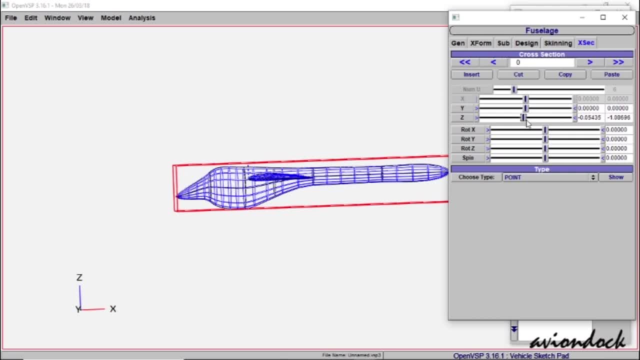 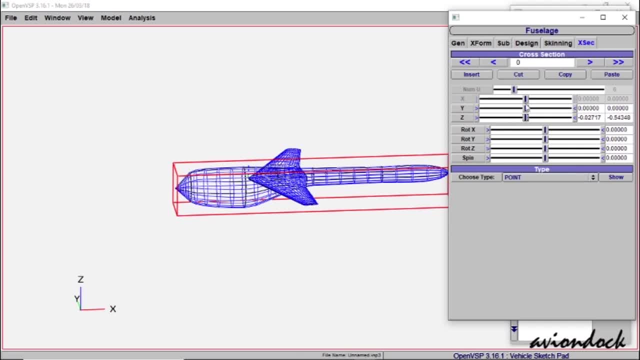 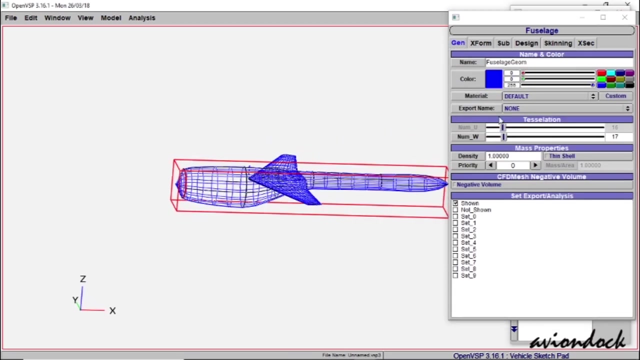 And not waste any more time in getting the very good geometry. Okay, I think this is all right for me now, And so probably we could assume that this is a tractor configuration UAV, where you have a propeller in the front and, yeah, let me move the fuselage a bit more lower down so that 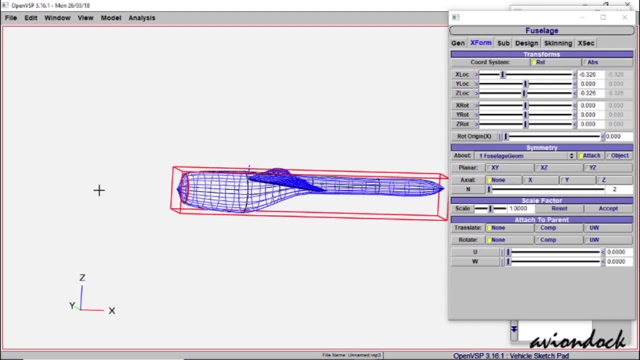 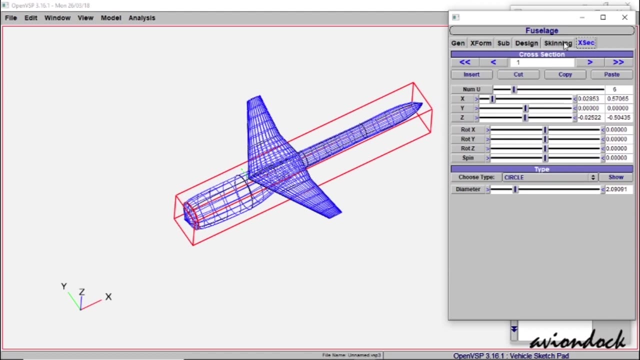 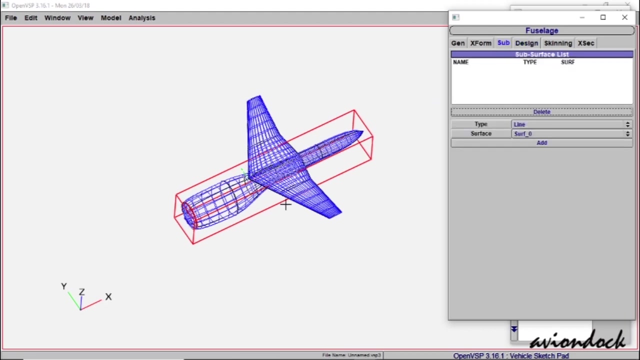 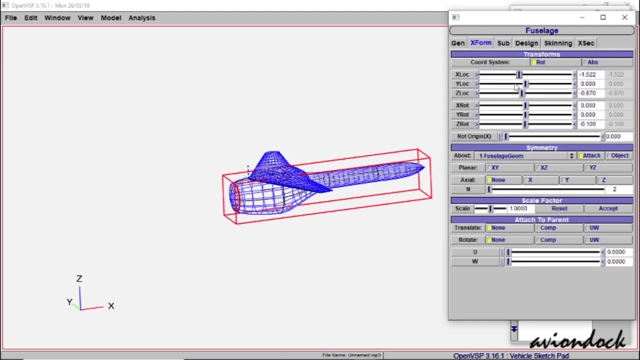 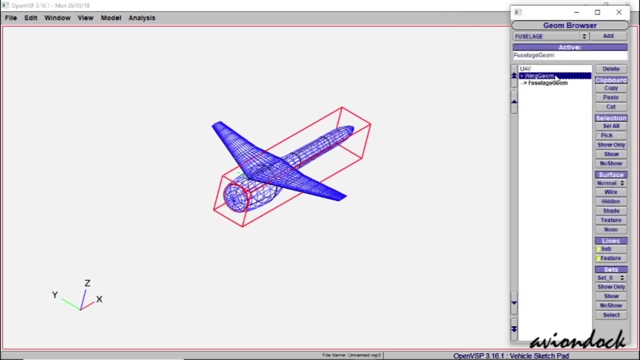 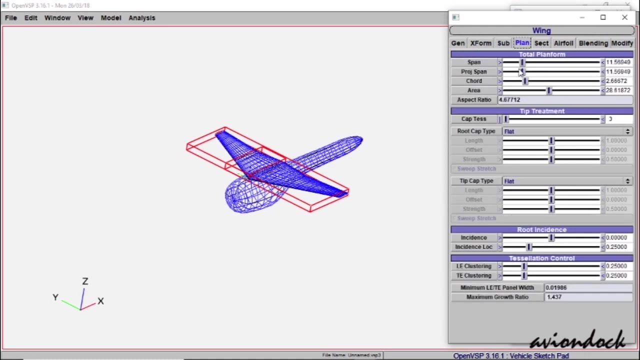 we have the wing as a high wing configuration. all right, that look good for now and also, overall, reduce the length. let me change this to 15 and move the reflection weight back. so just to keep the scales of various components same, i'm going to increase the span a bit of the swing. 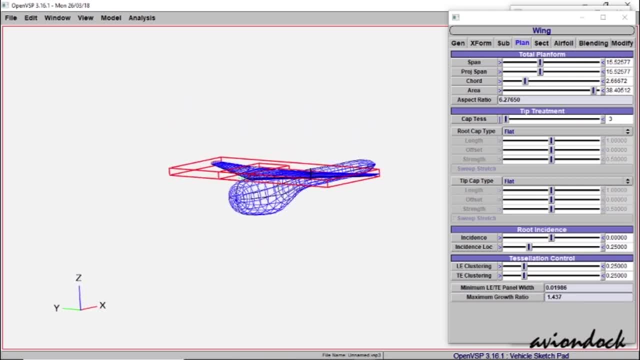 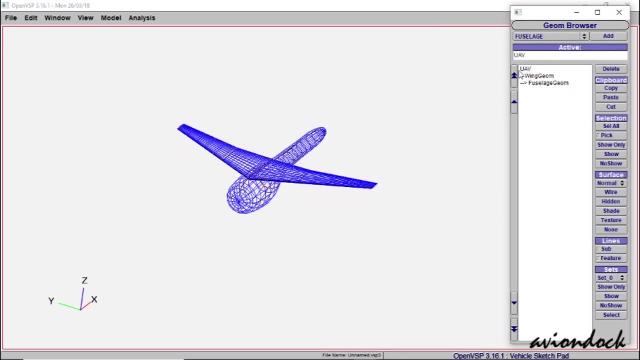 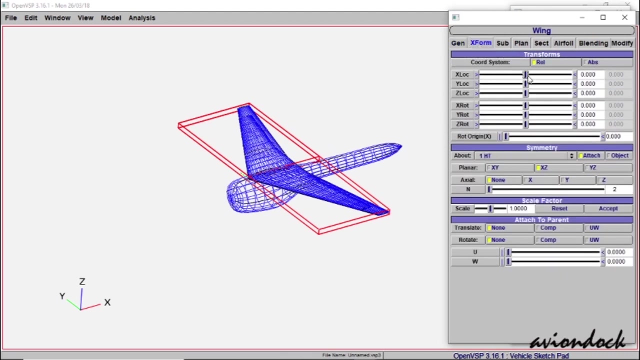 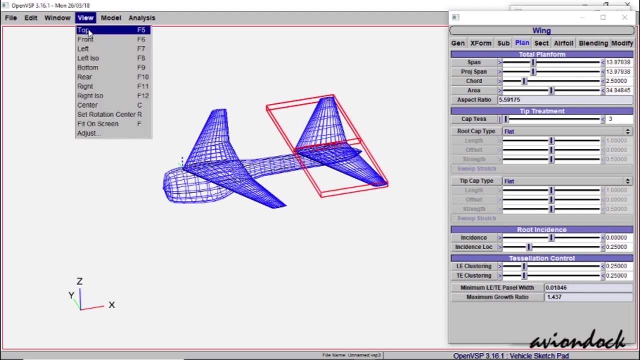 so that looks much better now. let me now add another wing, which is going to be our horizontal tail, so let's call this the hd or the horizontal tail- and we change the x location and obviously scale down the size, reduce the span, so you can always play around with the views to have a more appropriate control over. 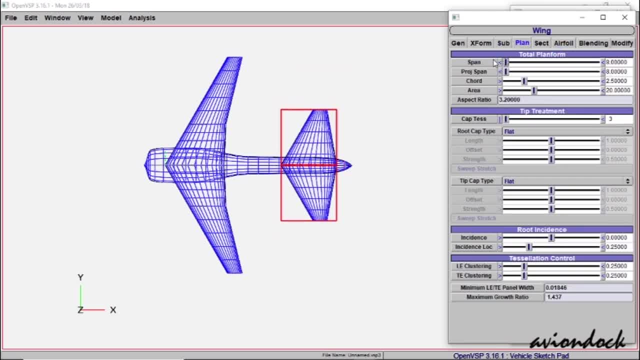 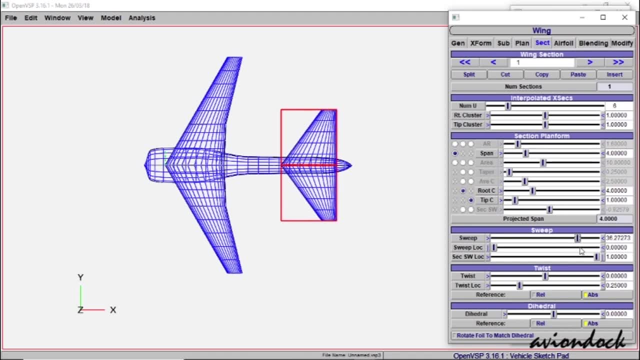 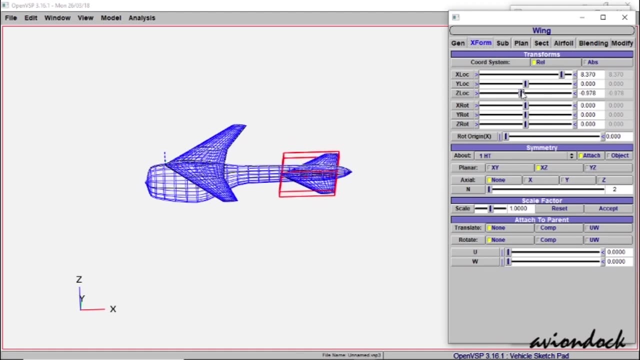 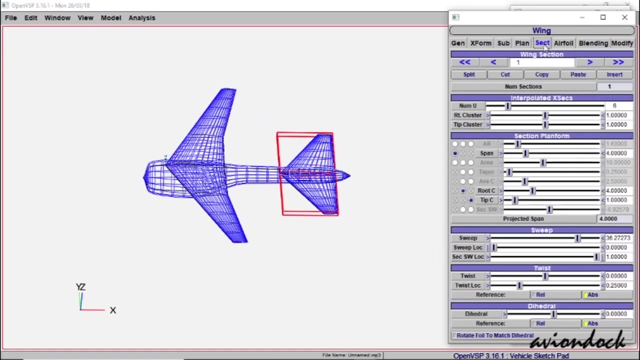 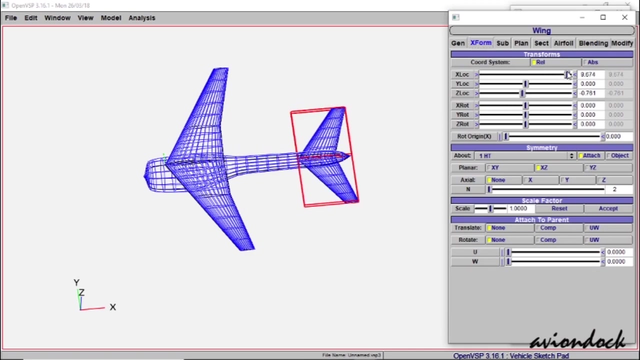 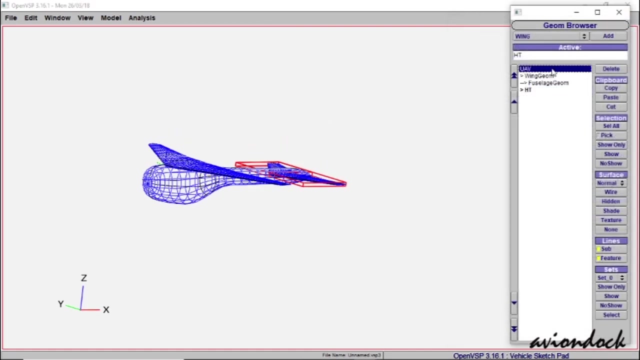 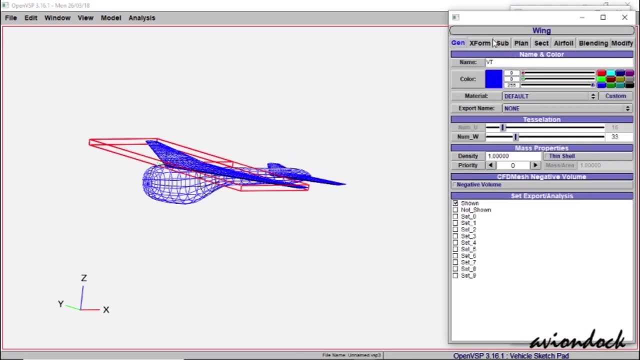 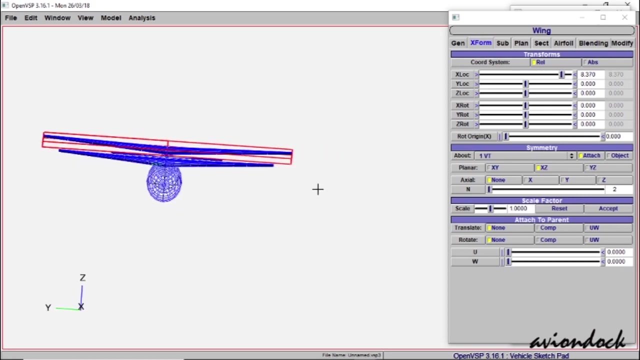 how the features are being defined. use the sweep section. so all right, that looks okay now. next, let me add vertical tail, so we name this vt and change the location. so what is important in the vertical tail is to have just one side of the wing and not a symmetric wing, so we can change that with the rotation feature. 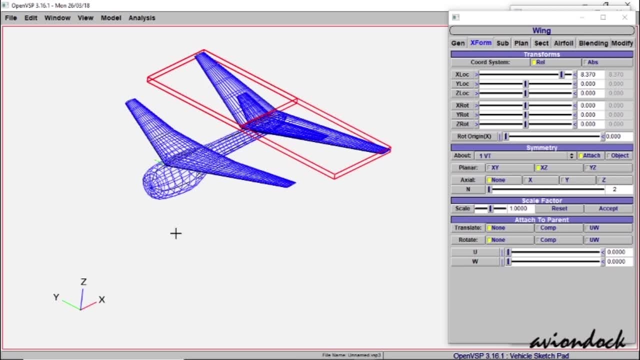 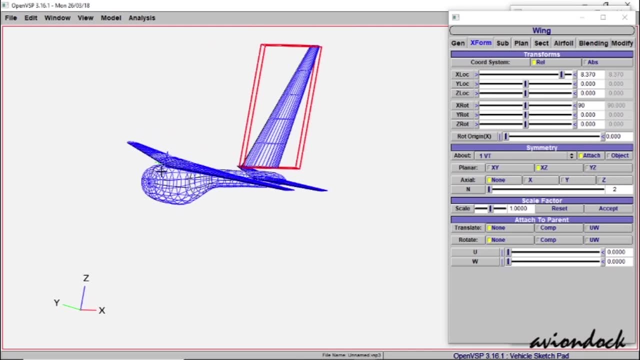 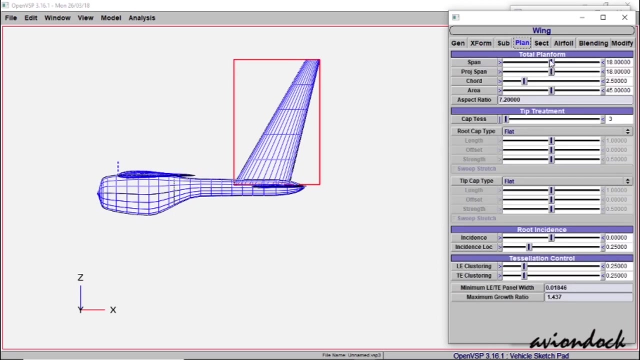 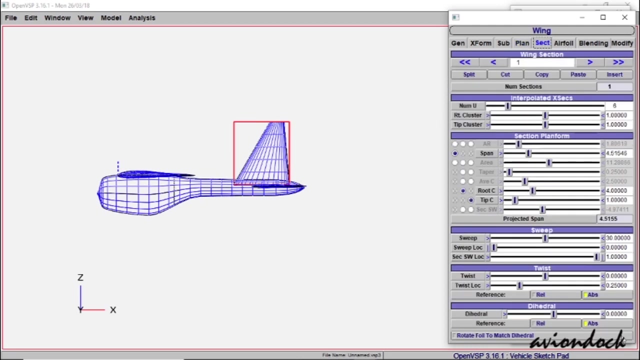 that is, we have this wing along the x-axis, so we rotate it along the x and change that to 90 degrees. there it merges into a single wing section which we can then modify. so let's reduce the span and sweep. it looks still oversized, so let me reduce that even more. 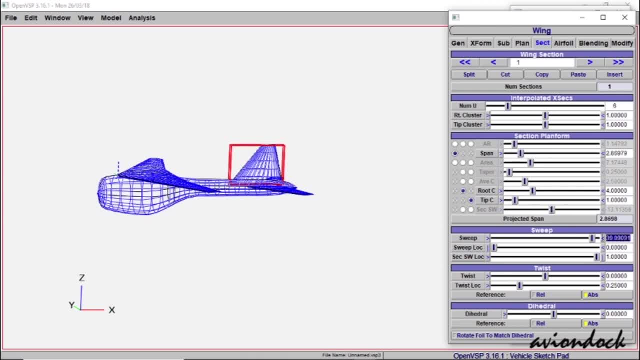 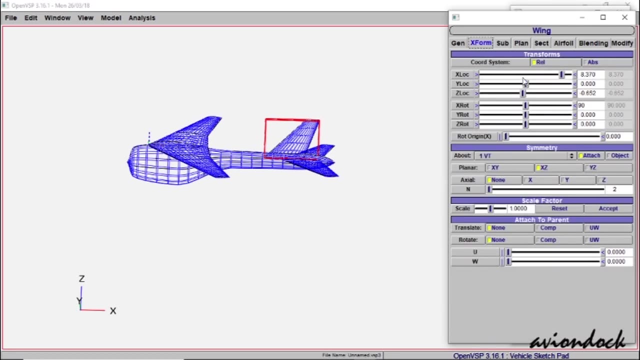 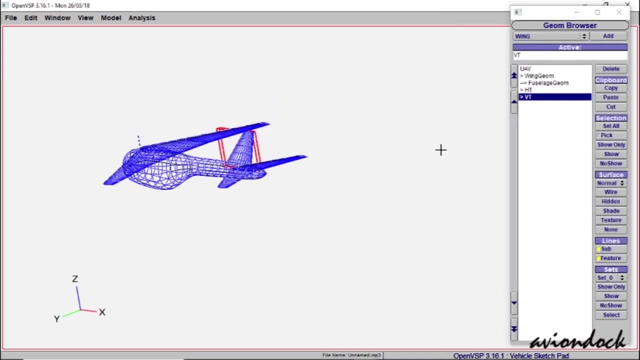 so you can see how this is working. so once you have the vertical tail right, you can alter the width to use anything you want, and let's go ahead and do the same thing with the vertical tail. so let's do that again. Again, we have not defined any pre-required mission or any particular wing loading. 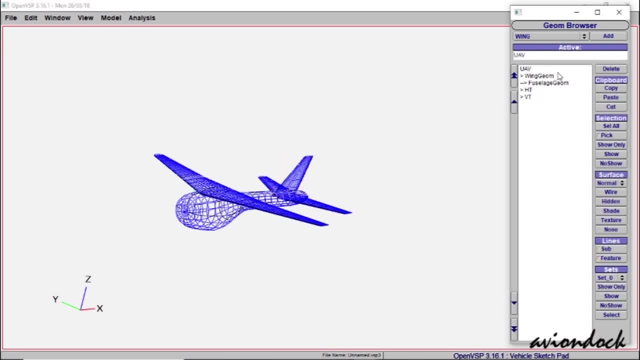 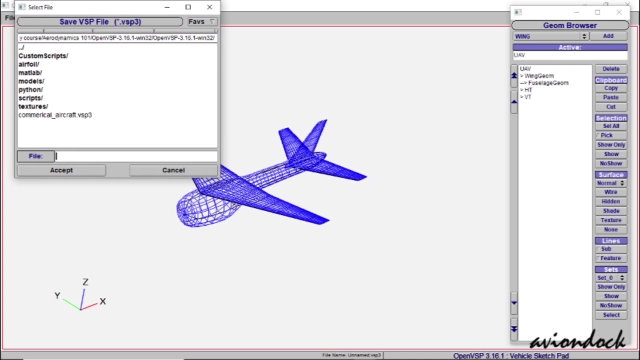 So this is just an arbitrary configuration for our analysis. So, having defined all of these parameters, let us now look at analysis. So here in the analysis feature, before that, let me just save the model and I call this UAV. So, under analysis, the first one we have is computation of the geometry. 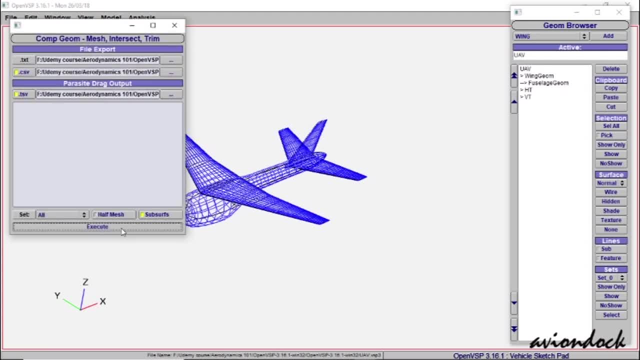 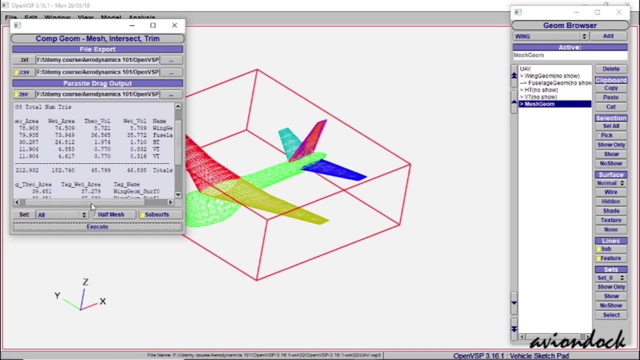 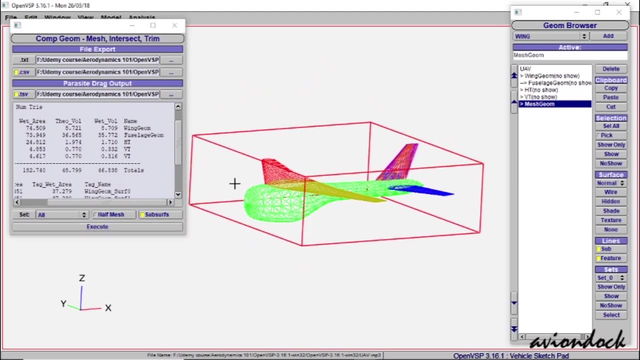 And so all we have to do is just click, execute and it computes the geometry. So what it does is it calculates the theoretical area and the wetted area for each of the components that we have used to make this UAV, And what we have to do is we have to calculate the theoretical area and the wetted area for each of the components that we have used to make this UAV. 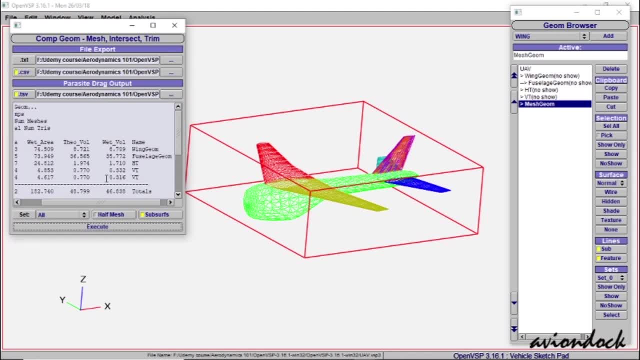 So why is this important? So the wetted area is an important quantity to be used in the parasitic drag calculation, So which we will come across later, and hence this calculation also tells us what is the total wetted area of the entire aircraft. 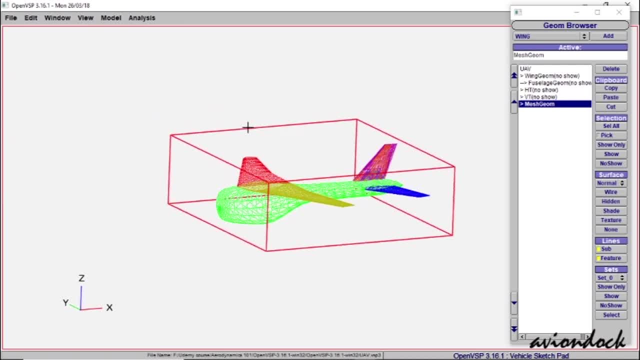 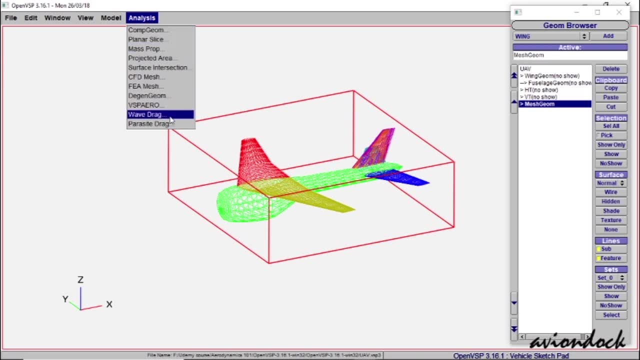 So once that's done, it also prepares the model for further analysis. Next let us go on to parasitic drag, Sorry. let's first look at degenerate geometry. So what degenerate geometry does is also that it creates new instances of the same configuration so that it can be used for other type of analysis, such as aerodynamic analysis and structural analysis, which require not just the outer shape of the aircraft but they require a panel configuration, for example for vortex lattice methods. 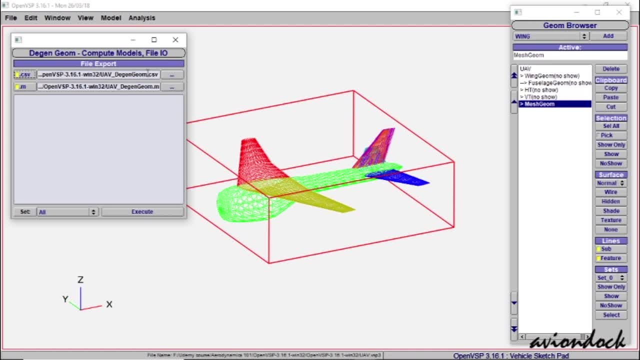 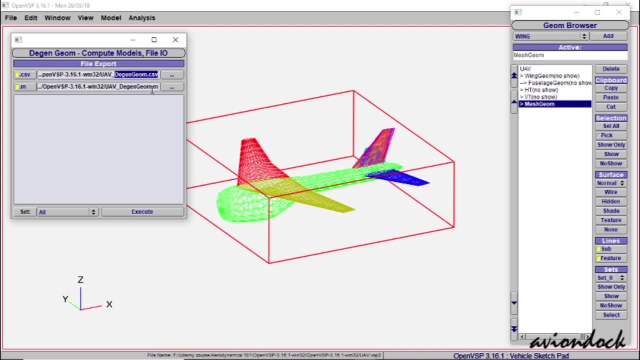 analysis in either MATLAB or in another Python script to perform optimizations or do any kind of structural load analysis or aerodynamic calculations. So let's just execute this, and it also shows you that two files have been created. Next let's look at parasitic drag. 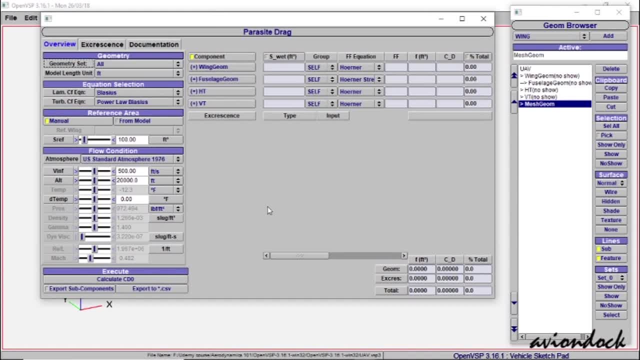 So parasitic drag is the drag that's not generated due to lift, but the drag due to the shape of the aircraft. So parasitic drag can be broken down into skin friction drag, industry drag and air drag. So if we look at the aircraft we can see that the aerodynamic drag is also generated due to lift. But the drag is not generated due to lift, but the drag due to the shape of the aircraft. So parasitic drag can be broken down into skin friction drag, Interference drag and pressure drag. Pressure drag is mainly due to the shape of the body and it's more dominant in the wake. 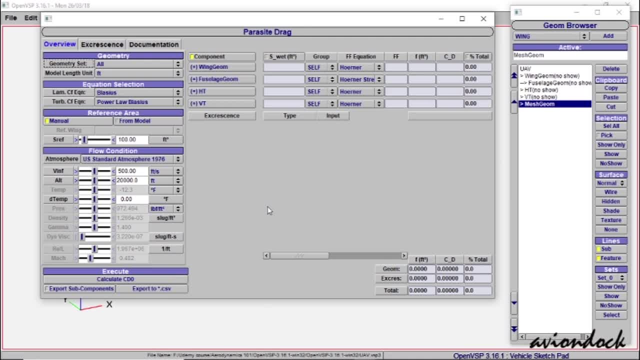 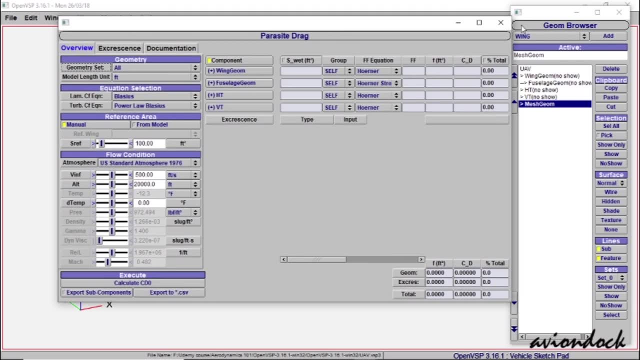 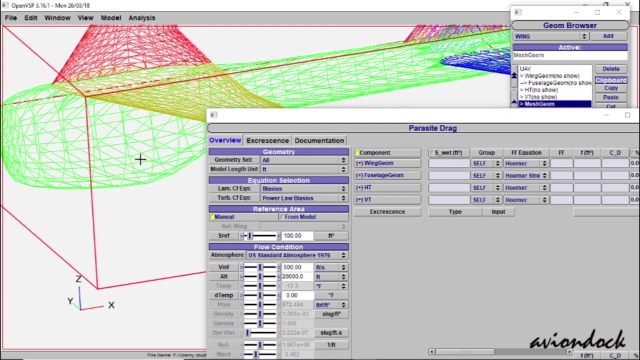 While skin friction drag is dependent on the wetted surface area of the body and the friction, because you have something known as the boundary layer that acts very close to the surface of the aircraft, and And So you have something known as the no slip condition, where the fluid sticks to the surface and 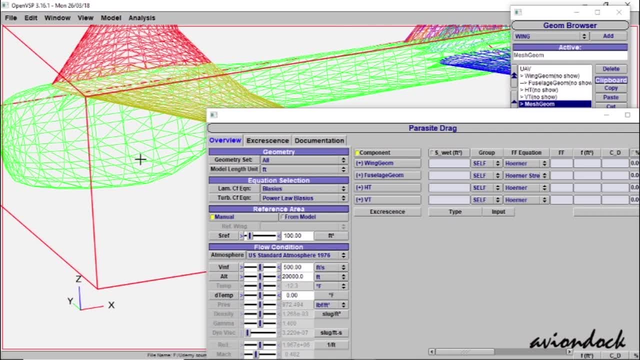 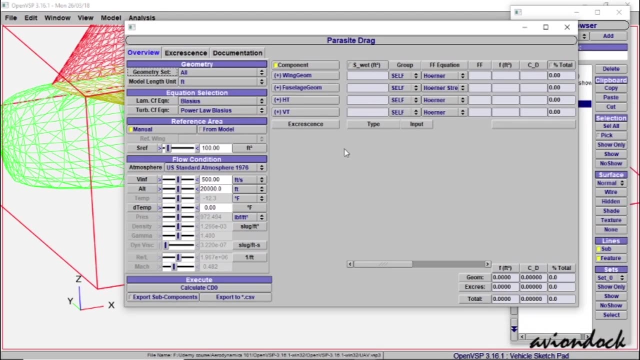 There is a gradient of velocity that you see within this boundary layer. Now, this boundary layer can be laminar or turbulent, and they can create different magnitudes of the drag. so what we do here in parasitic drag is to use some kind of a handbook method to 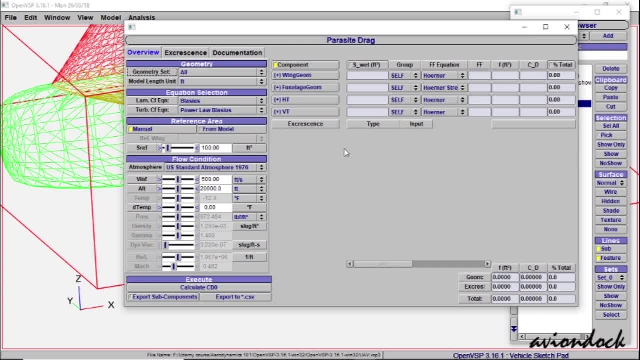 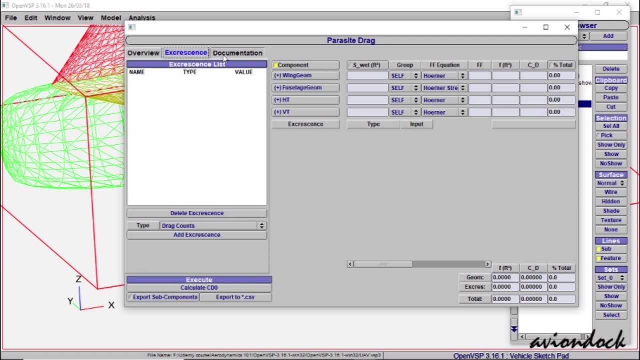 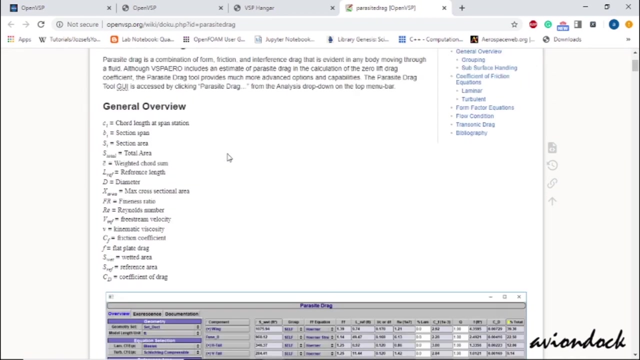 Compute what could be the estimated parasitic drag contribution of the entire aircraft. so to learn more about the types of equations that's being used, you could go to the documentation tab and Click on the link to the complete wiki. So here we see the instruction manual for how the parasitic drag tool works. 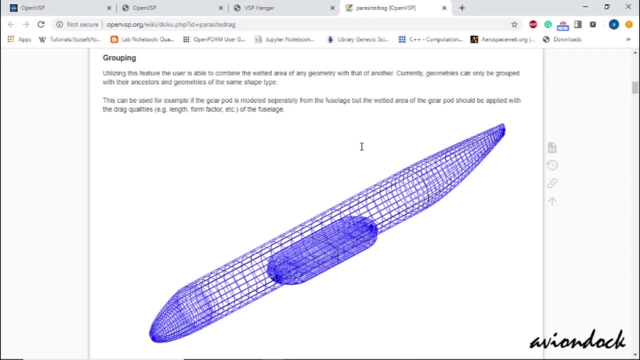 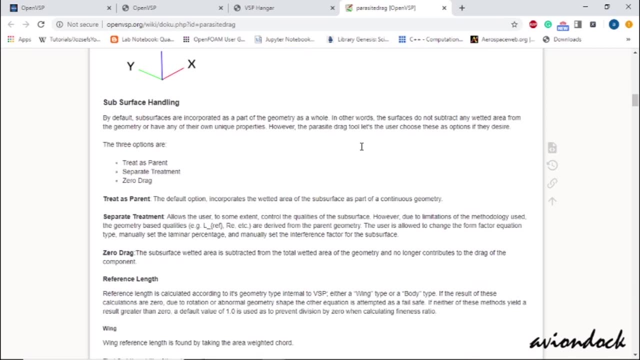 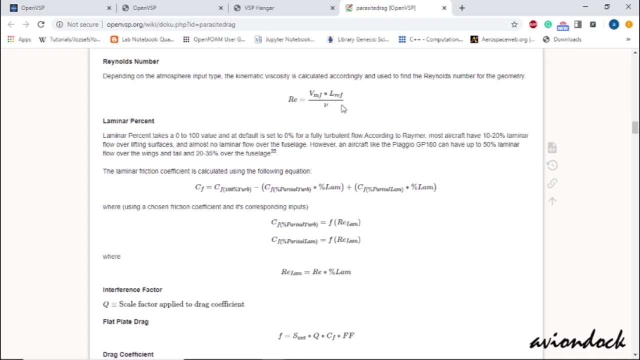 So it's pretty much easy to follow along these Theory that's given here. Why? how does the software calculate the wetted area, How does it deal with surface intersections and Calculating the Reynolds number of each component, and also predicting the right formula to be used for. 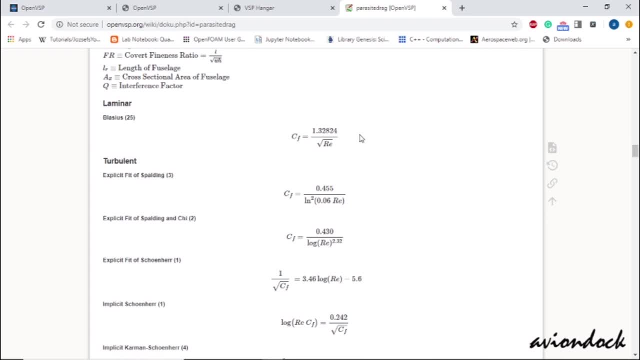 Both the laminar skin friction and the turbulent skin friction. so there are various methods of estimating the skin friction, which is a function of the Reynolds number. so, based on experimental data or any pre-existing aircraft models as a reference, you could choose the correct turbulence and the laminar model for 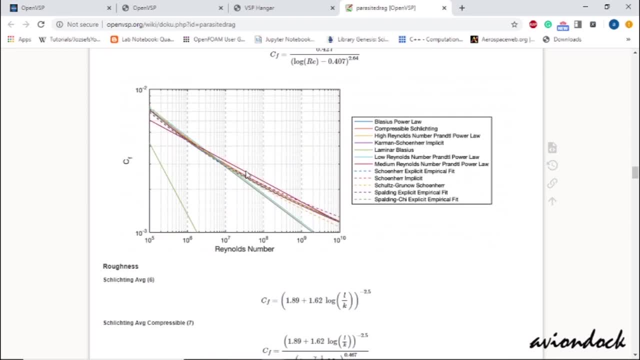 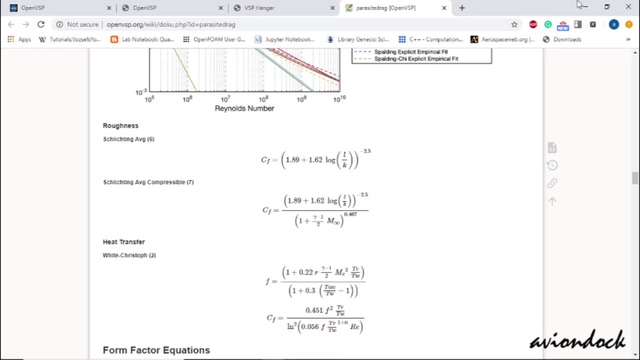 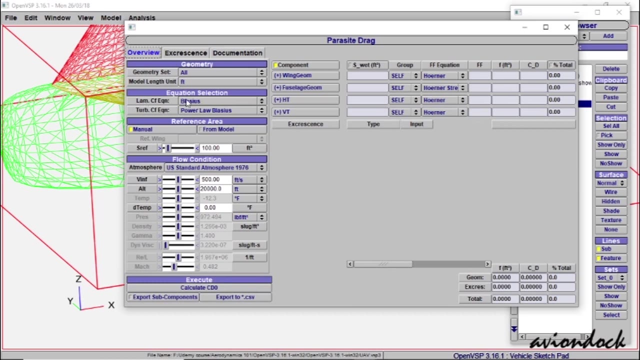 your skin friction drag calculations. here we also see the magnitude of skin friction variation with the Reynolds number. so here I'm going to leave these as default. so it says that it's going to use the blesses equation for the laminar skin friction calculation and the power lobe lashes for the turbulence skin. 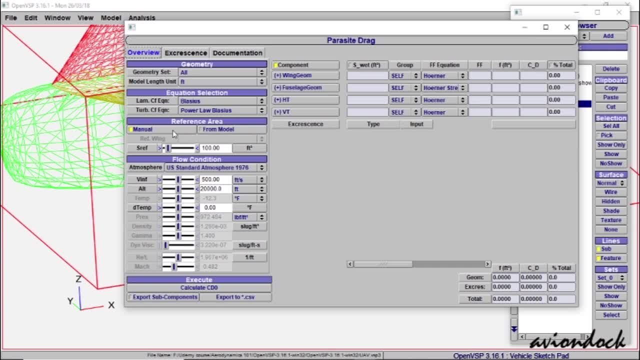 friction calculation. next we look at the reference area. so any kind of non-dimensionalization of the drag coefficient is based on a reference area and that reference area is based on the direction that the drag coefficient is area is usually taken as the wing area. so here we set it from the model and 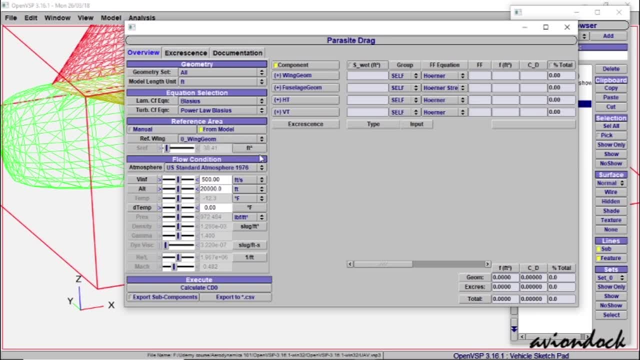 refer that to the wing geometry and also set some operating conditions. you can change the units by setting the right dimensions here, and then we can change this to our liking. let's just set the free speed of 200 meter per second and 8,000 meter altitude, and so here we have the wing components. so when I click, 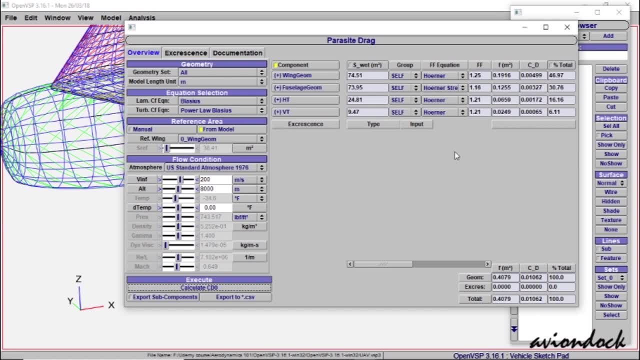 calculate CD not. you see these colors being filled up. so what open VSP does is use the wetted area calculated from the previous option that we just carried out, that is, to degenerate to geometry, and use that to also find out what is the form factor contribution. 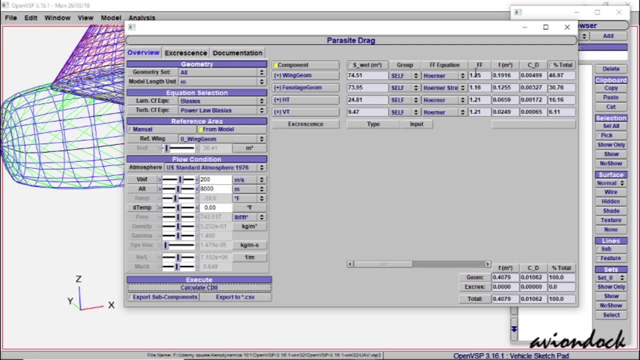 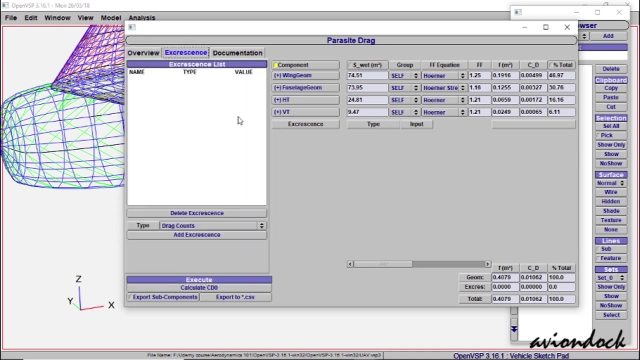 and all of these parameters, such as the skin friction and the form factor, summed up together gives you an estimate of the final drag coefficient. so here we see that the total drag coefficient, that is, a parasitic drag, is 0.01062, and another interesting variable that we see here is Xsense. so since it's a very basic model, 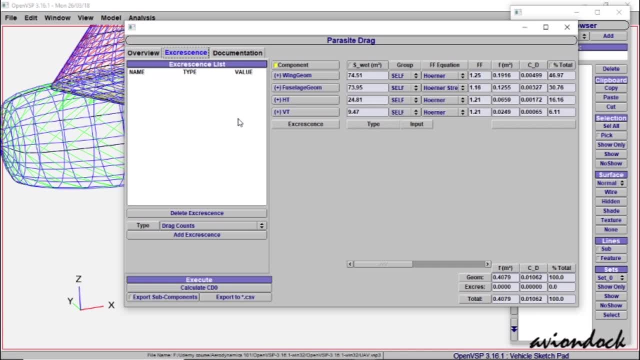 you haven't accounted for windows or any kind of projections or känh surface irregularities, such as sensors mounted on the exterior of the aircraft, landing gear, etcetera, so you could just add a rough additional value. so let me just take that as 10% of the total drag. 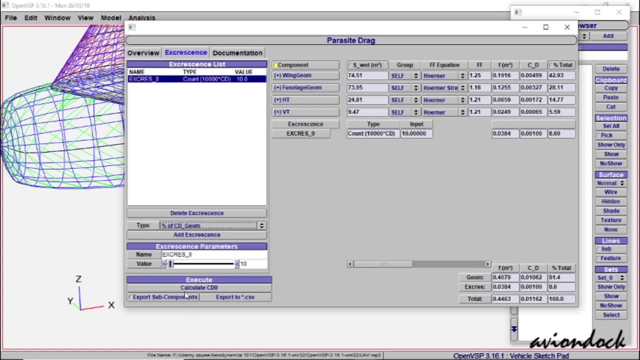 coefficient and recalculate the CD zero. so here we have thehelplae drag aldered, which is around 10% of the total drag, and there we have the new value of the parasitic drag coefficient at 0.01162.. So it's also interesting to see the breakdown of the drag. 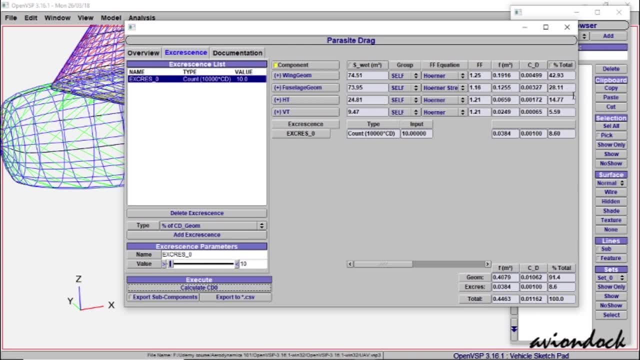 contributions from the various geometries. So we have the wing at 42%, followed by the fuselage horizontal and vertical tail. So any kind of modifications in order to reduce the parasitic drag might be focused more exclusively on the wing and the fuselage geometry. 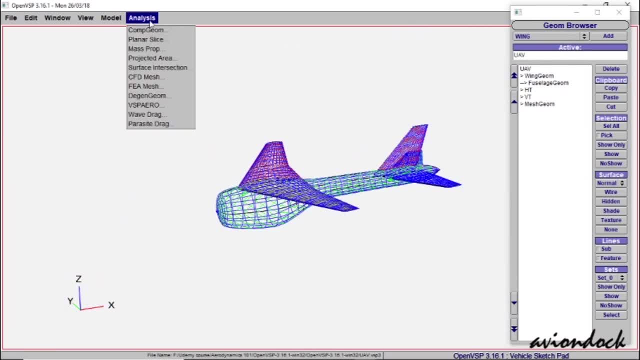 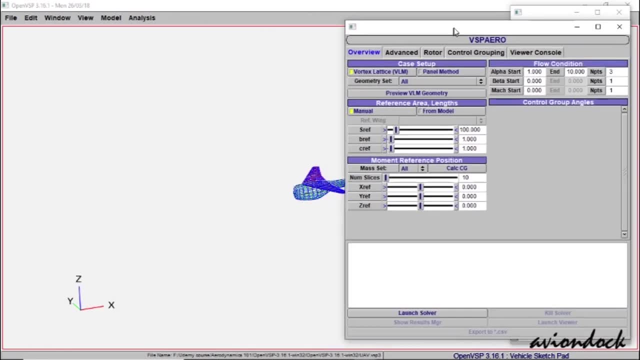 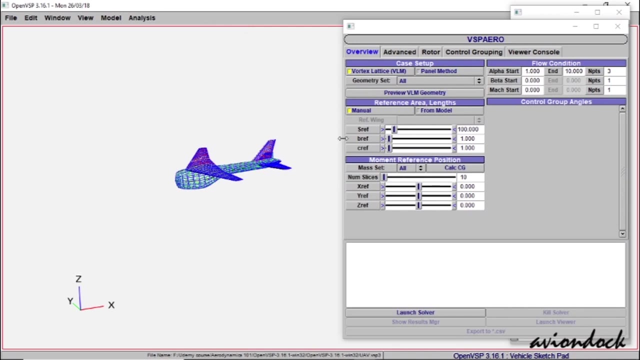 Since we have parasitic drag out of the way, let us now go to an aerodynamic analysis. So in the aerodynamic analysis, OpenVSP uses two different methods, So that is the vortex lattice method and the panel method. You can read up more about these methods online, but rough understanding. 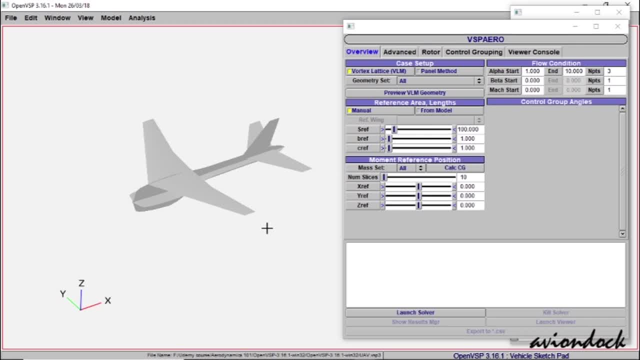 and use of these methods will be discussed in the next video. Thank you for watching. can obviously read up through this in any aerodynamic textbook. but to just get running here, we start with the vlm method, and what vlm cannot do is to predict. 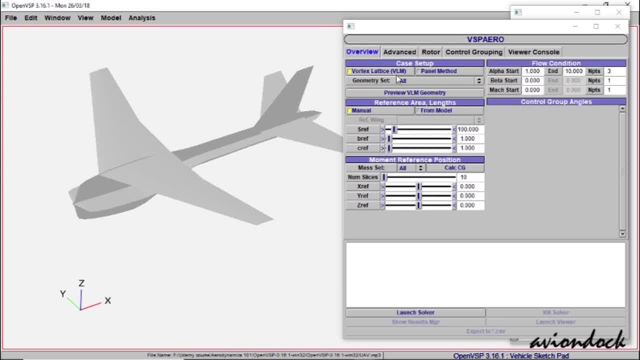 any kind of viscous feature of the flow. that is, it doesn't take into account the boundary layer that's been created. so in the parasitic drag calculation that we carried on earlier we do account for the skin friction and the interference drag and overall account for the boundary layer of the aircraft. but here we look at the entire flow. 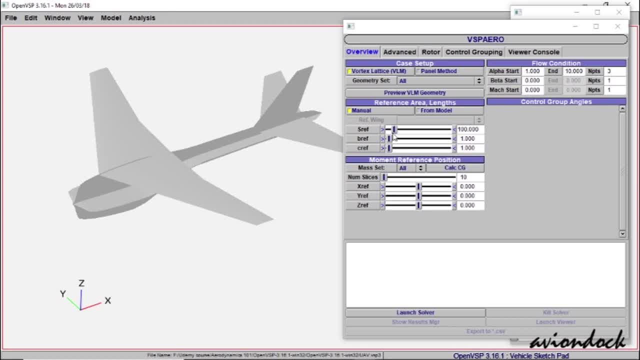 as inviscid, that is, the absence of viscosity. so what is the disadvantage of this feature is that we cannot see any kind of non-linearities in the aerodynamic measurements of the lift and drag quantities, and there is also no prediction of flow separation from the bodies, which which 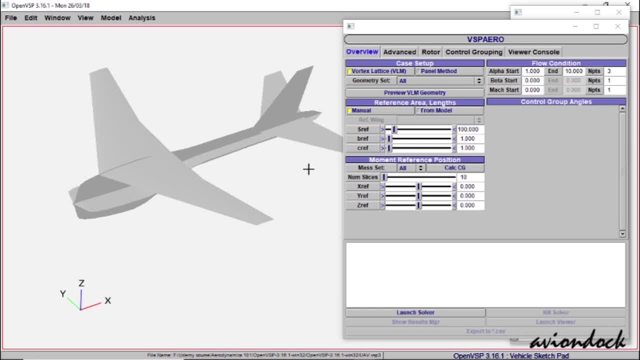 restricts us to a very high flow rate of the aircraft, So this is a very interesting feature. However, in conceptual design, we actually do not require an extensive, in-depth insights into the fluid flow around the body, because eventually we're going to carry out flight tests or use. 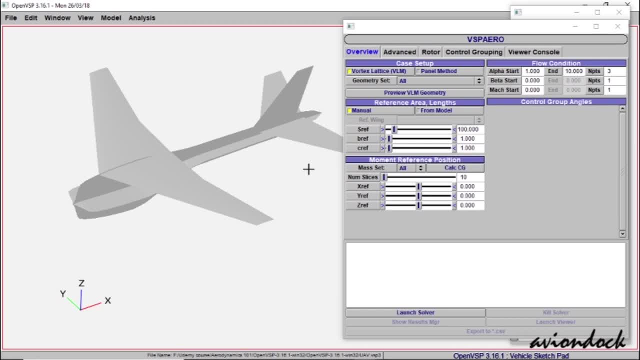 wind tunnels or computational fluid dynamics to further refine the aerodynamics of the aircraft. So let me set the reference area again to the wing geometry, and here we have the flow conditions. that is the angle of attack of the aircraft. so let me just send it from. 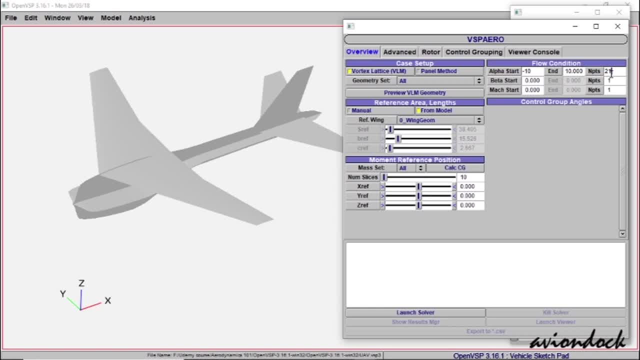 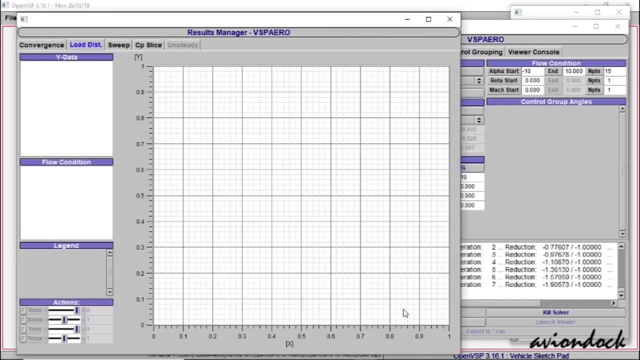 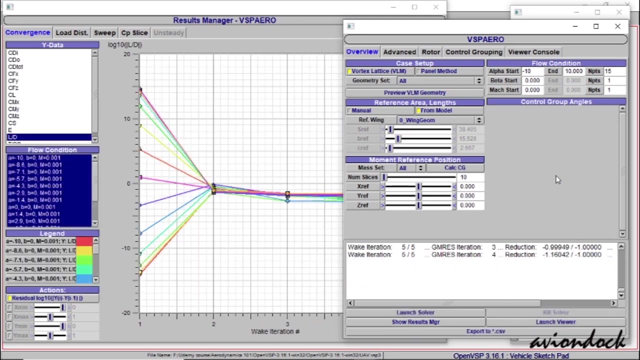 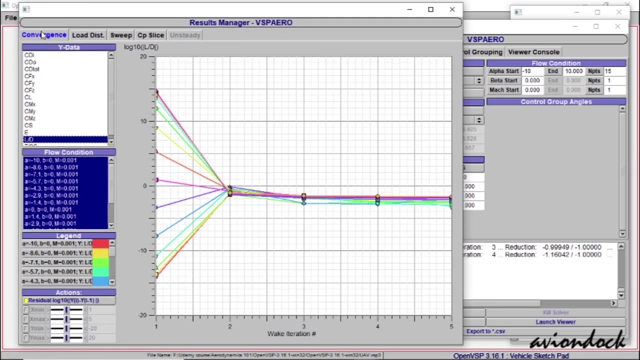 minus 10 to positive 10 degree and set up, let's say, 15 points, and that's all that's required to perform an initial run and we launch the solver and then I'll show you the first tutorial I'm going to do. Alright, so the calculation has been completed. so when the results manager, what we see is first convergence plot, that is, there are multiple iterations that the solver uses to allow the solution, and here we can see that it has taken five week iterations and our solution has converted in this way. 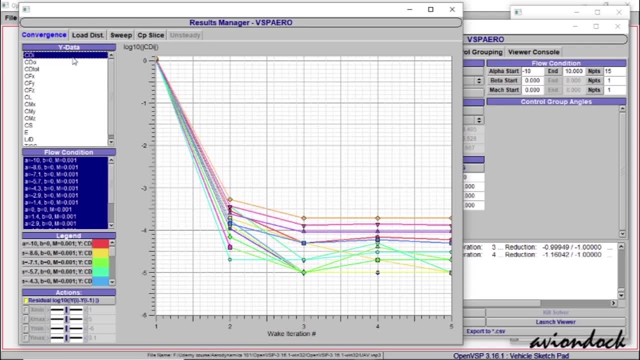 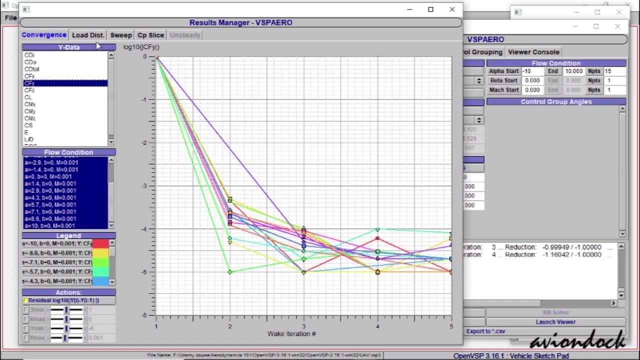 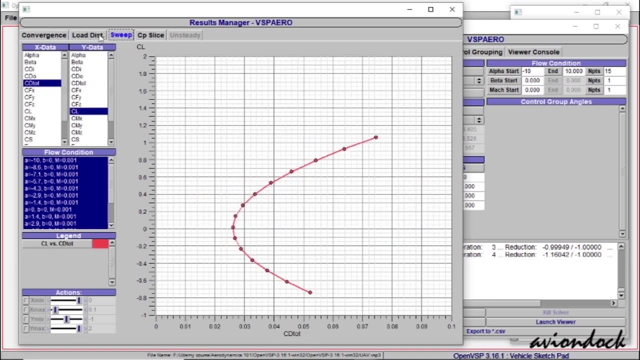 to a stable value. you can also check this for other parameters, such as drag coefficient or the vertical force. so let's look at load distribution and we can see. sorry. let's first look at sweep, and the most interesting thing to look at is the lift coefficient versus angle of attack, and you see that with an 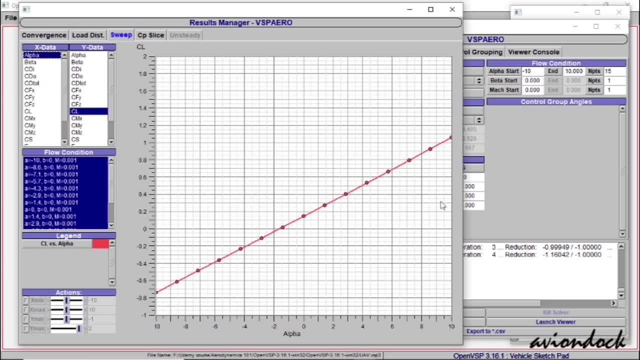 increase in angle of attack, you have an increase in lift coefficient, and let us next look at the induced drag versus lift coefficient, and this is a very important graph that we would require in order to figure out what is the induced drag contribution for the lift coefficient at which the aircraft cruises. 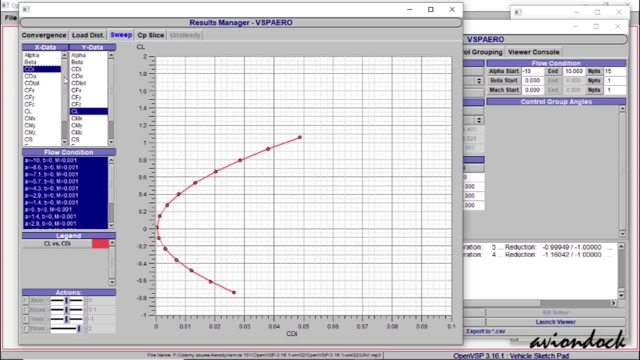 so, since I previously told you that the VLM is unable to calculate the parasitic drag, the induced drag coefficient is not the only drag coefficient that we are interested in, so let us also look at CD 0 and the CD total. so when you add the parasitic drag, 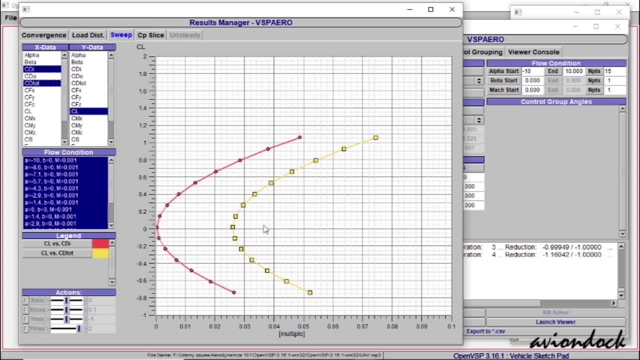 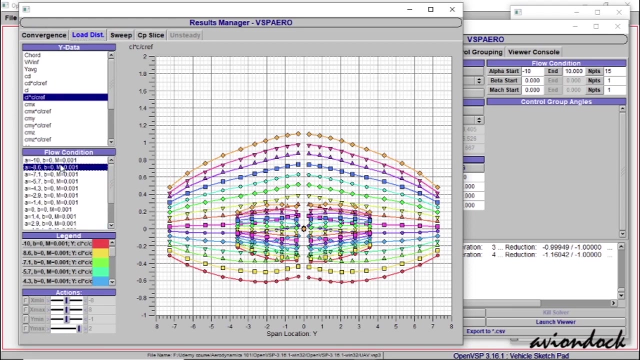 to the induced drag, you have a much higher drag coefficient, corresponding to lift coefficient, and this would give you important information such as the angle at where you fly at minimum drag and also the kind of propulsion system that would be most efficient for this configuration. so in the load distribution you can also see the span wise distribution of the.